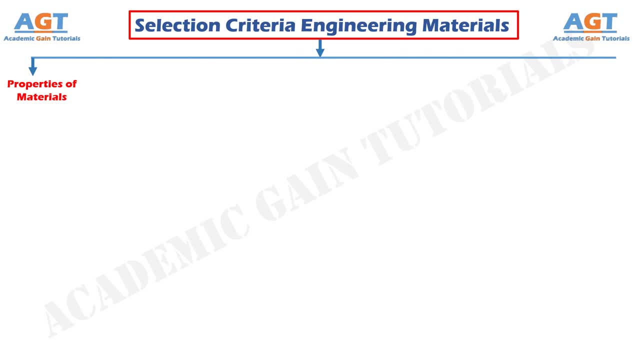 1. The Properties of Materials. It is the most important factor. The properties of material define specific characteristics of material and form a basis for predicting the behavior of the material under different conditions. The important properties of materials are: Mechanical, which includes stresses. Thermal, which denotes heat or cold. 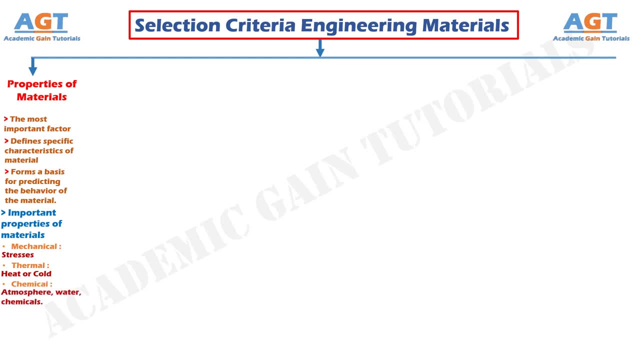 Chemical, which includes change in property of materials with change of atmosphere, water chemicals. Electrical, which includes change in property of minerals with change of the state of the matter, power and current. and radiation, which includes light, ultraviolet, nuclear performance requirements. the material of which a part is composed of must be able 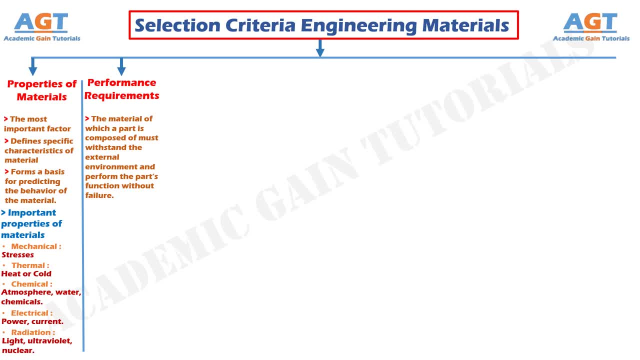 to withstand the external environment and perform the parts function without failure. for example, the material of a furnace wall must withstand the high temperature. we also need to consider the materials reliability in a given application. a material must be reliable. reliability is the degree of probability that a product and the material that the product is made of will remain stable. 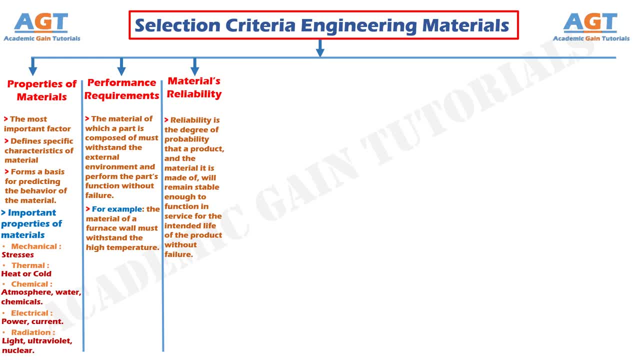 enough to provide service for the intended life of the product without failure. another important factor to consider is safety. a material must safely perform its function, otherwise the failure of the product made out of this material may be catastrophic in certain situations, such as in airplanes and high-pressure systems. 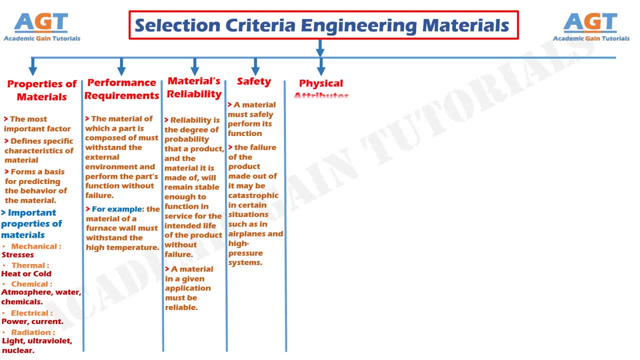 physical attributes. the physical attributes, such as configuration, size, weight and appearance, sometimes also serve as the functional requirements. for instance, the functioning of a gyroscope or a flywheel is directly related to the weight of the material used. environmental conditions: the environment in which a product operates strongly influences service performance. 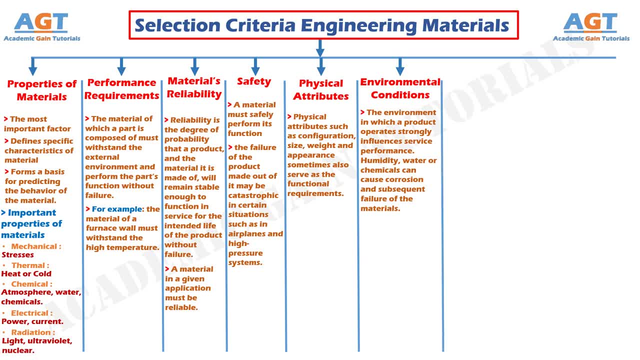 humidity, water or chemicals can cause corrosion and subsequent failure of the materials. availability of a material: obviously a material must be readily available and it should be available in large enough quantity for the intended application. in times of scarcity, this becomes significant factor of consideration. disposability and recyclability: these are the highly significant and